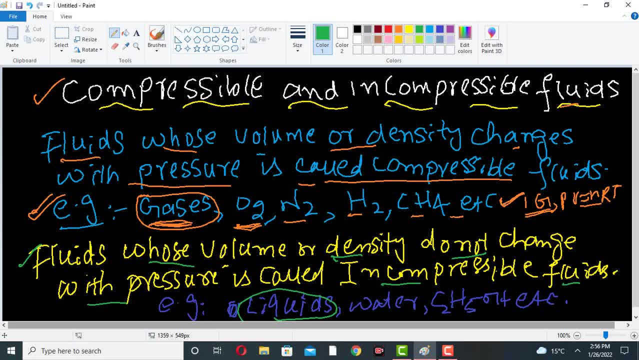 For example, liquids. Liquids are called incompressible plumes because their volume do not changes with pressure. Liquid like oxygen, Liquid like water- ethanol, methanol, ether, etc. are called of some petroleum diesel. These are the incompressible plumes. 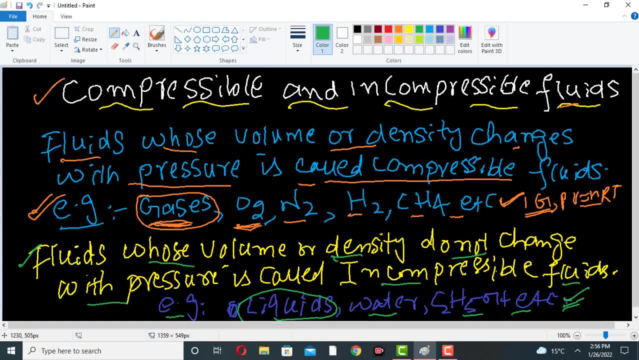 So the main difference between compressible and incompressible plumes is that the volume or density of compressible plume changes with pressure, But the volume or density of incompressible plume don't change with pressures. So this is the main difference between compressible and incompressible plumes. 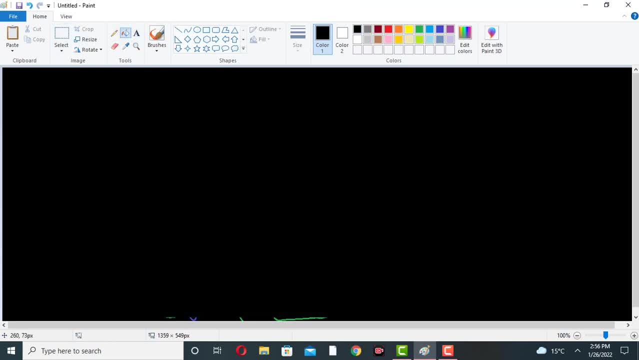 pressures. so this is the main difference between compressible and incompressible blue. so now there are some. for example, if you draw, the key you draw for the compressible tools like this is the volume and this is the pressure. so the when we increase the pressure on gases, then their volume will be decreased, like this: 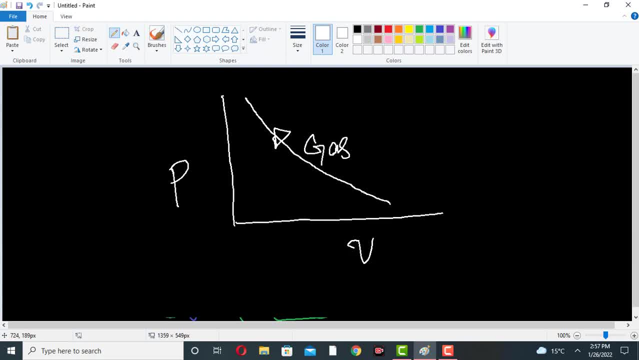 so this is the. gases are the compressible fluids. so, similarly, if you draw the key, you draw for the. this is the volume, this is the pressure, so the. if we increase pressure on the liquid, then their volume will be slightly decreases or it will be very. there will change in volume, the pressure will be. 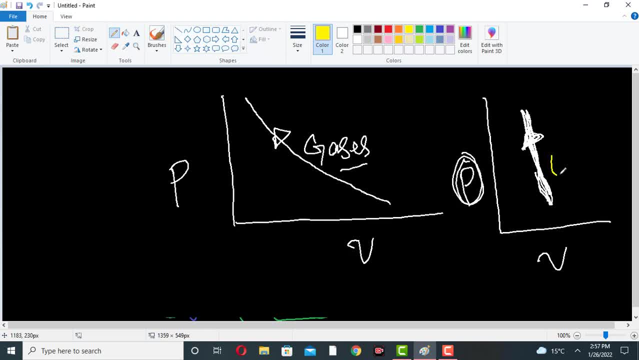 ignored. so this is the liquid. so liquid is incompressible because incompressible because the volume of liquid may slightly decreases or changes with increase in pressure. so consider to be incompressible but the gases, but the gases, that the volume of gases decreases with increase. 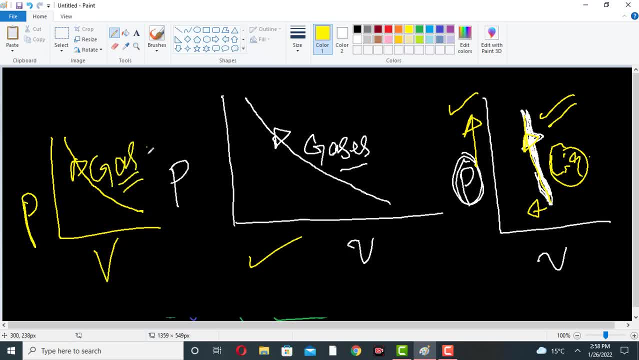 in pressure, so this is considered to be compressible. so this was a small difference between the compressible and incompressible fluid. so this was a little difference between compressible and incompressible fluids. thank you very much for your attention. if you are new to the channel, please like and subscribe to my channel. thank you very much.